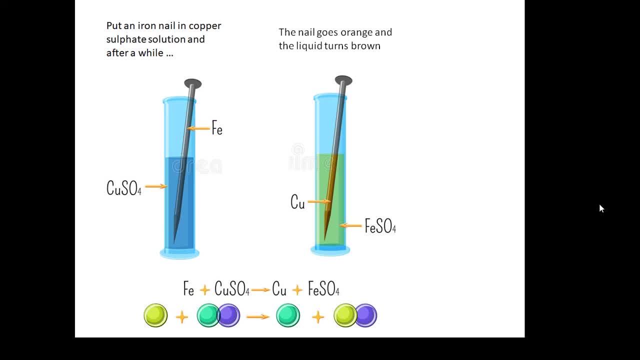 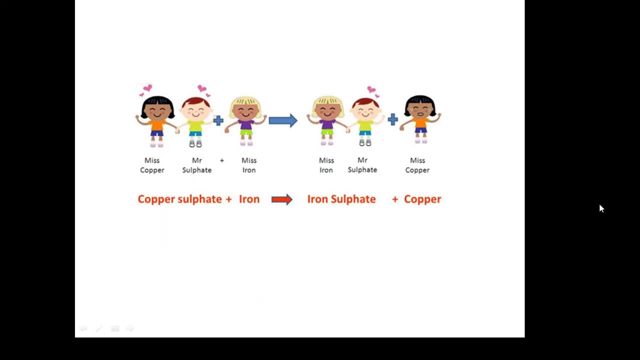 place of the copper, and the copper has been kicked out, It has been displaced. Okay, and this is a displacement reaction. Looking at this, there's copper, sulfate, the happy couple. Miss Iron comes along and she pinches Mr Sulfate. Okay, and you end up with Iron Sulfate, the happy couple. 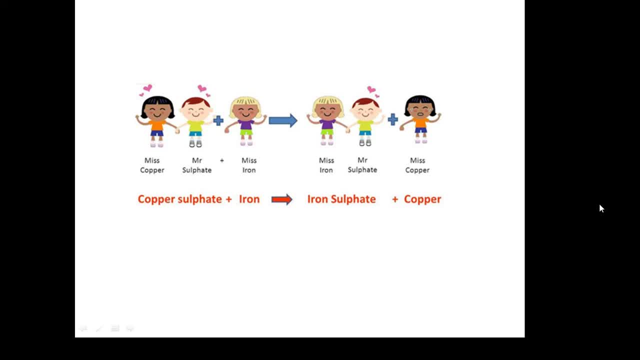 and Miss Copper has been kicked out. Okay, that's the way it goes. So copper sulfate plus iron goes there, Iron Sulfate plus copper, and that is a displacement reaction. Now, a displacement reaction will only happen if the metal involved at the start is more reactive. Okay, So for example, magnesium plus copper sulfate. Yes, Because 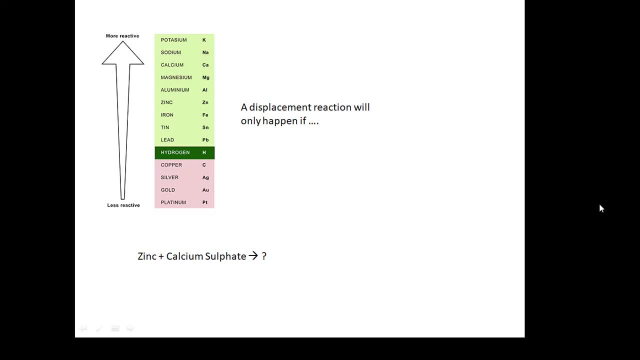 magnesium is more reactive. Iron plus copper sulfate: Yes, Because iron is more reactive than copper. zinc plus calcium sulfate: no, nothing's going to happen. okay, because zinc is less reactive than calcium. so you look at these and tell me: will there be a reaction? if there is a reaction, then what will the products be? uh, or will there just be no? 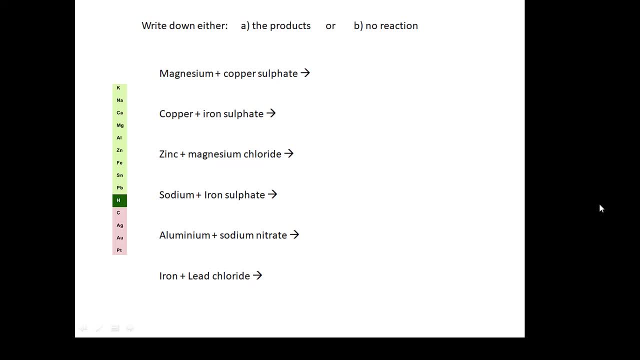 reaction. okay, notice, by the way, on this reactivity series. uh, carbon is there. that's interesting. we'll come back to that later. fluorine, chlorine, bromine iodine- what group is that? what is this group called? hopefully you recognize this is group seven and it is the halogens. yes, group seven. 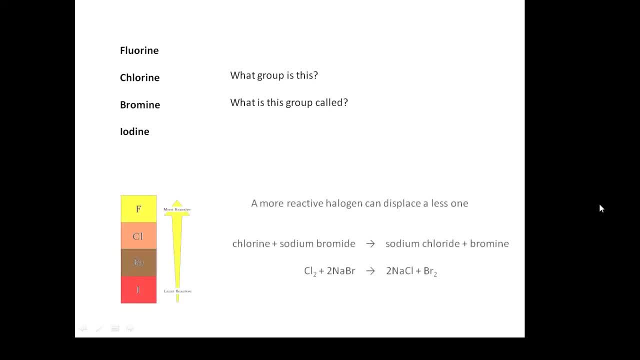 now they can do a bit of displacing as well. okay, a more reactive halogen can displace a less reactive one. for example, chlorine plus sodium bromide will give you sodium chloride plus bromine. okay, the chlorine is more reactive than the bromine and it can displace it. so halogens. 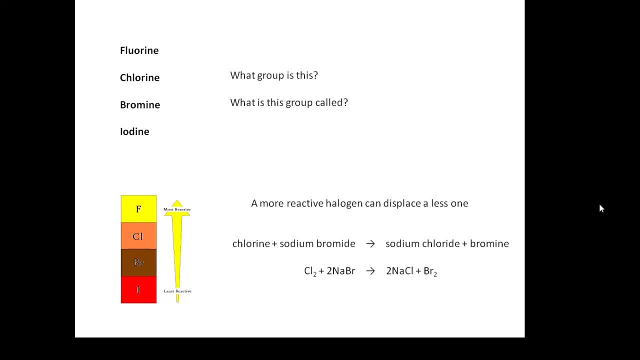 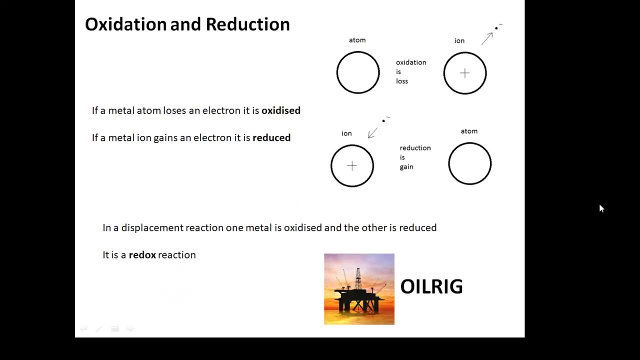 can be involved in displacement reactions as well. notice, however, the difference is that reactivity goes upwards. with the halogens, fluorine is the most reactive. so oxidation and reduction. now, in a lot of these reactions what we've seen is an ion becoming an atom and an atom becoming an ion, a metal atom losing an electron or two electrons. 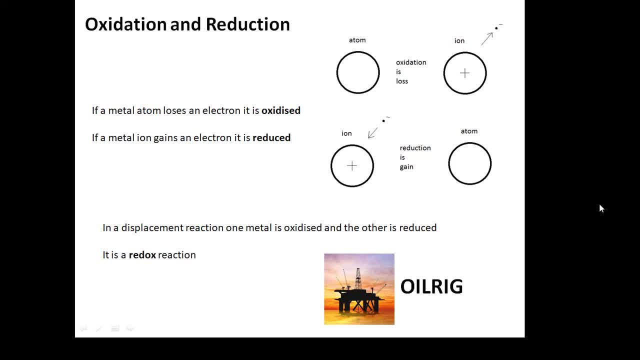 is an ion, and when this happens we say it has been oxidized. when an atom, a metal atom, loses one or more electrons, we say it is oxidized. so oxidation is loss of electrons. and then when an, an metal ion, gains one or two electrons, we say it is reduced. okay, so reduction is gain of electrons. 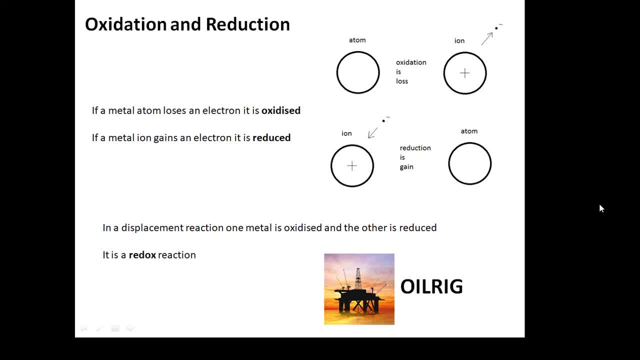 if a metal atom loses an electron, it is oxidized. if a metal ion gains an electron, it is reduced. there's one way of remembering this very useful: oil rig. oxidation is loss, reduction is gain, oil rig. okay, so in a displacement reaction one metal is oxidized and the other is reduced, for example in: 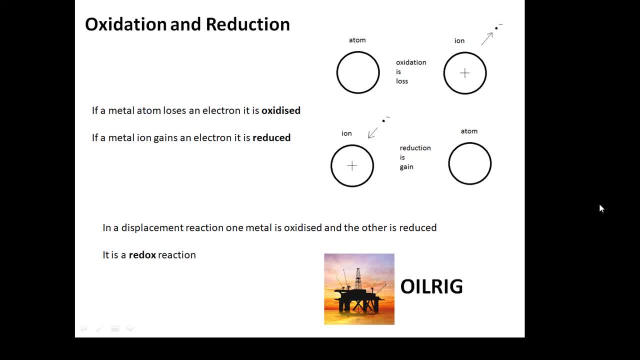 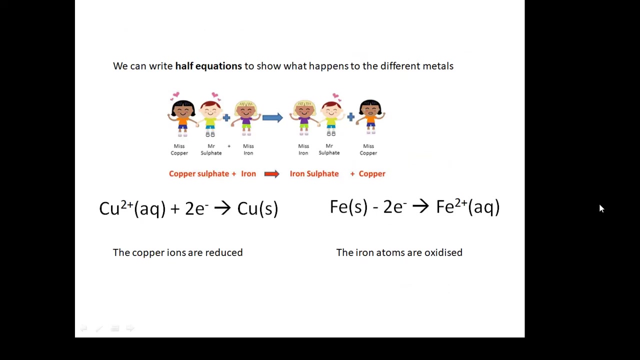 iron and copper sulfate. our iron atoms are oxidized and our sulfate, our copper ions- beg your pardon- are reduced. so oxidation and reduction. it's an example of a redox reaction, because you get reduction and oxidation happening. what we can do for these metal atoms and ions is write. 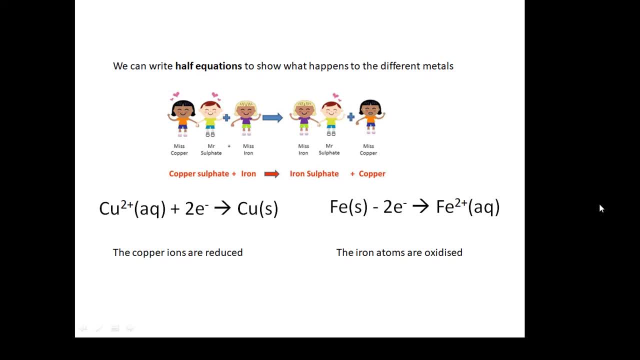 something called a half equation, and this shows what happens in terms of electrons, but just to the atom or the ion. okay, see you, two plus plus two electrons becomes copper. yeah, the copper ions are reduced. Fe minus two electrons becomes Fe 2 plus the iron atoms are oxidized and these are called.